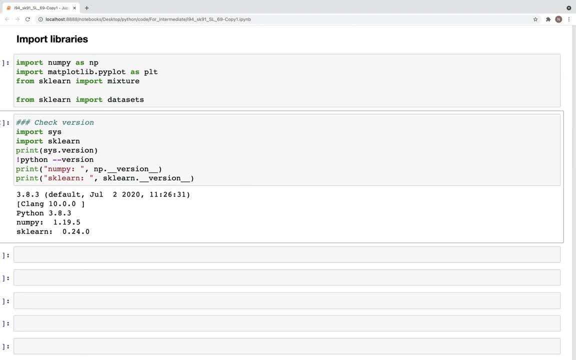 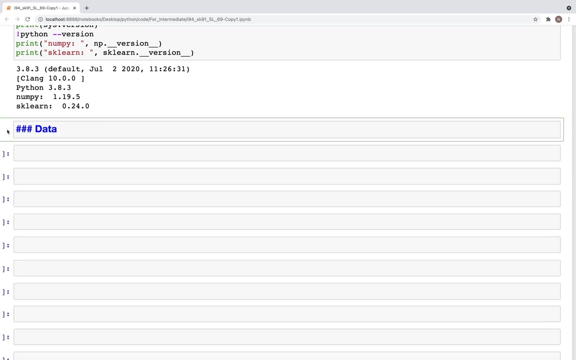 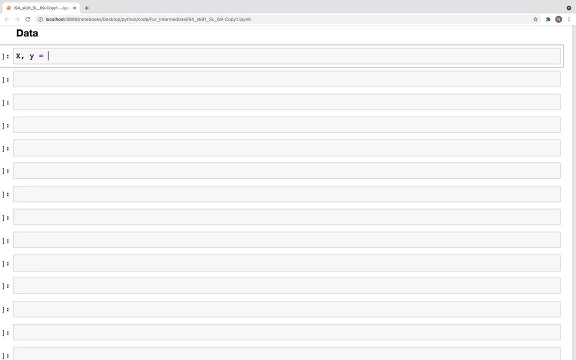 Here in Jupyter Notebook I've imported these libraries and these are the versions that I'm using. We need the mixture library, which is for the Gaussian Mixture models. For data. we'll use the iris dataset because it's simple dataset, So to get that we can type x, comma. y is equal to. 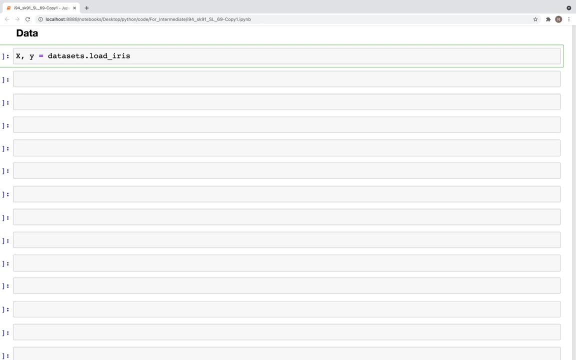 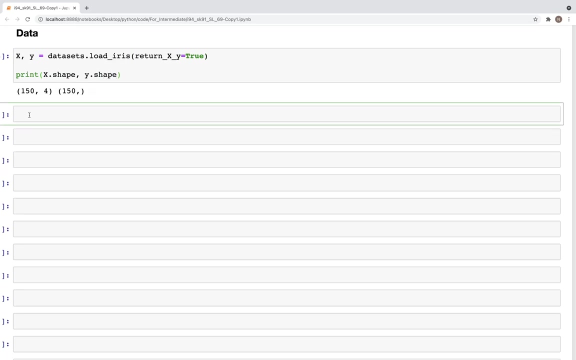 datasets: dot load: underscore iris, and here we can specify return: underscore x, underscore y is equal to true And we can print the shape of x and the shape of y. Those are the records that we have. We can plot this as well. So let's say x, zero is equal to. for plotting what we are going to. 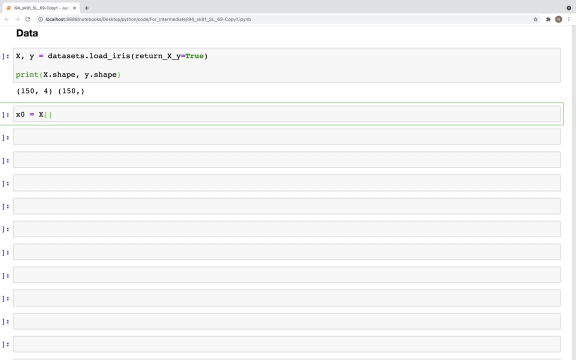 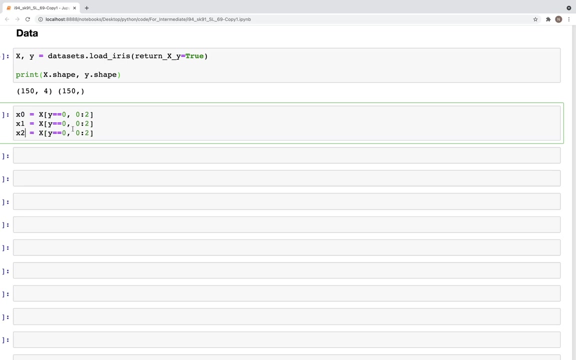 re-split this into different sets. So x, where the values for the class is 0, we set this to. y is equal to 0 and we'll pick only the first two columns and not all the columns. Similarly, we'll repeat this for x1, x2 and this could be one and this. 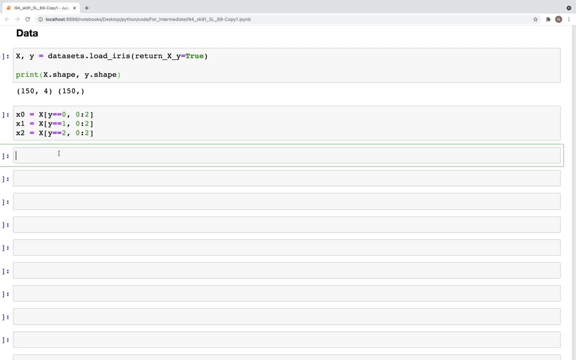 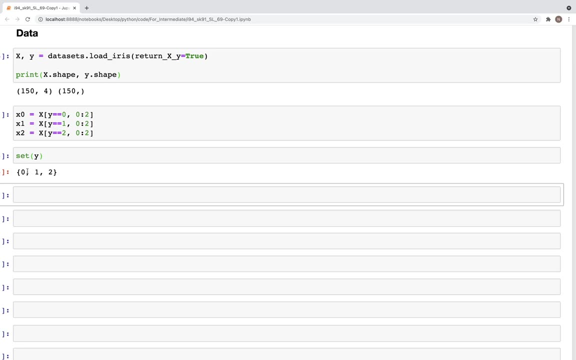 could be two. The reason why I've put one, 0, 1, 2 for y is, if you look at the total types of labels for y, it's 0, 1 and 2.. Now, I know that this is a label dataset, but what we are going to do is we are going to ignore the 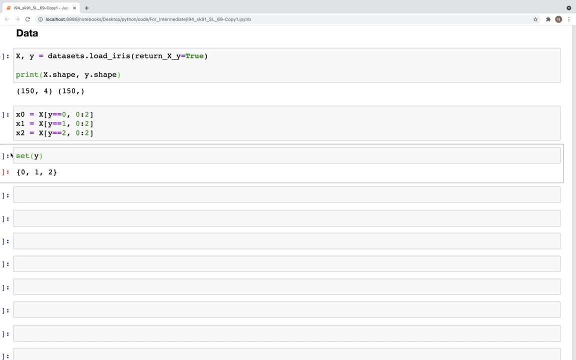 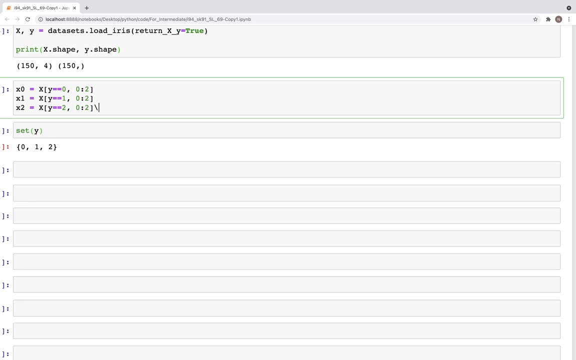 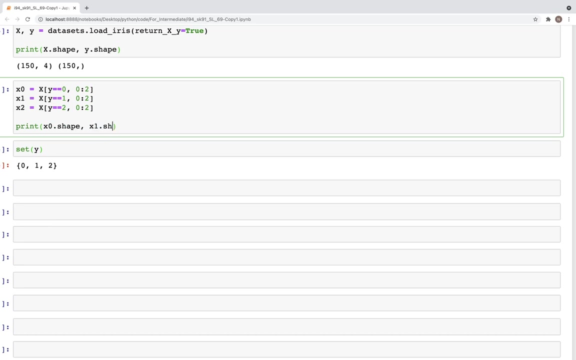 labels when we are training on Gaussian mixture models, but then use those labels to see how the clusters look after we perform the unsupervised learning on those models and we can so look at the shapes here. print x 0 dot shape. x 1 dot shape. x 2 dot shape. 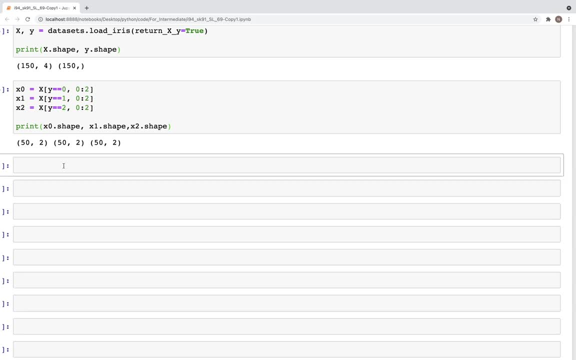 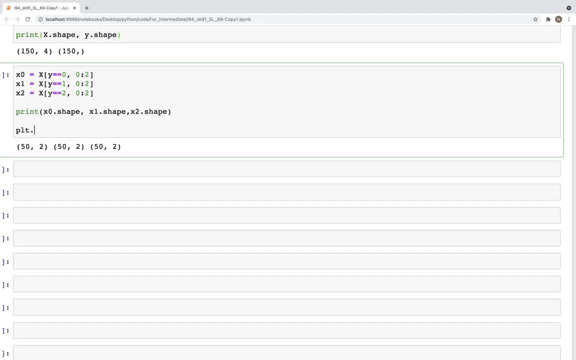 and we have around 50 labels in each of those columns. and finally, while we are at it, we can print our sorry, plot them so plt, dot, scatter x 0. and this is where we are going to have one column on the x-axis and then the 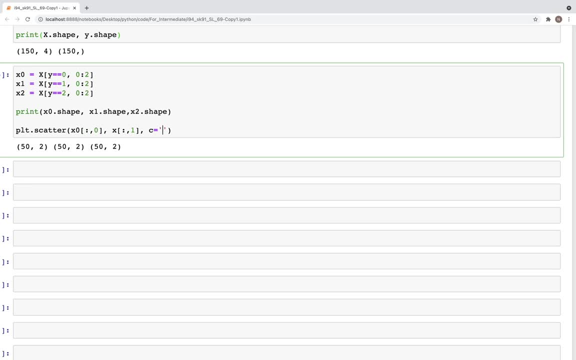 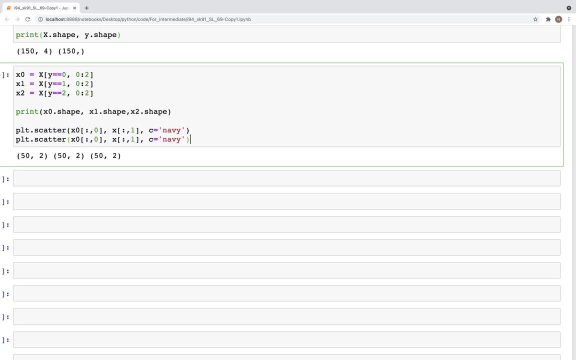 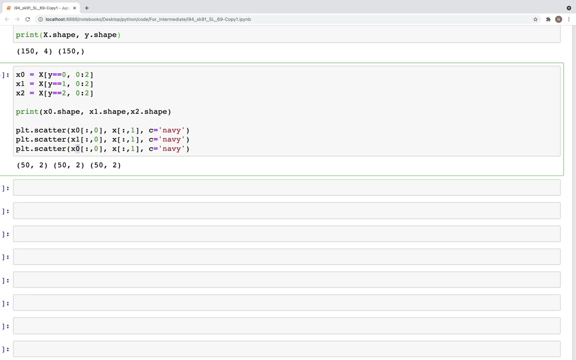 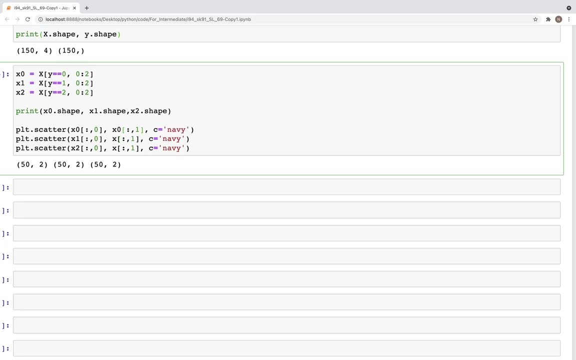 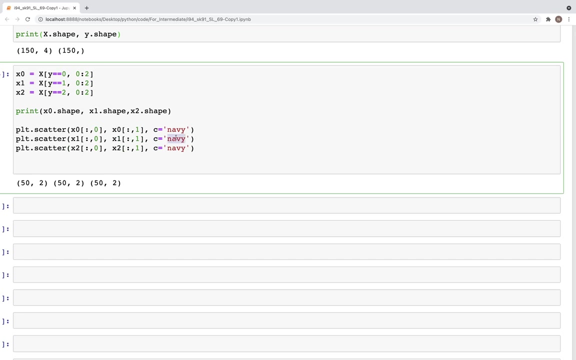 second column on the y-axis, and we'll specify the colors because we, when we plot the results from the unsupervised learning, you would need to specify the same colors there so that we can easily compare the two. so this would again be x 0, this would be x 1, this would be x 2 and then, if we can change this to, let's say, a green color and 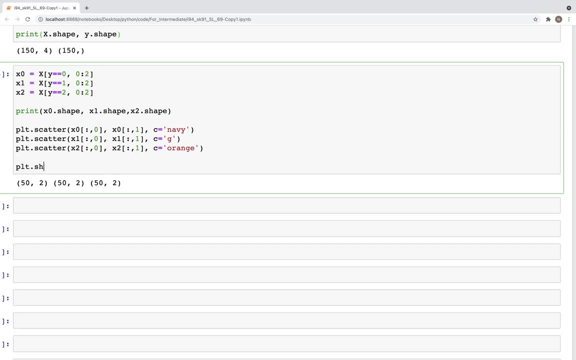 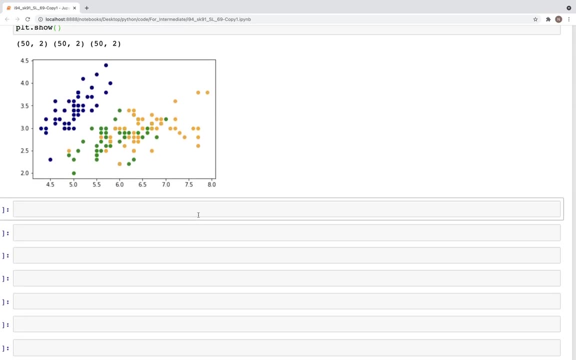 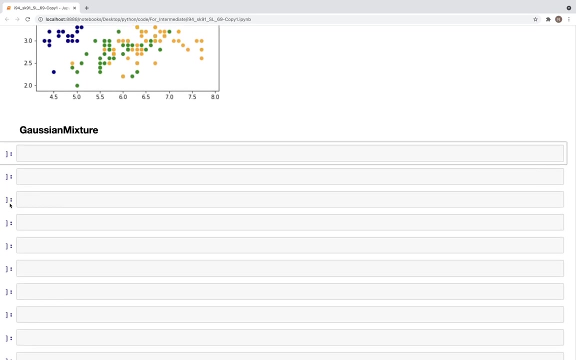 maybe an orange color and we can pop on purity dot show. so that's how the clusters are and let's see if the Gaussian mixture models are able to find them. so the very first one we'll try is Gaussian mixture, and this is without the Bayesian thing. so here we have: gm is equal to mixture dot. 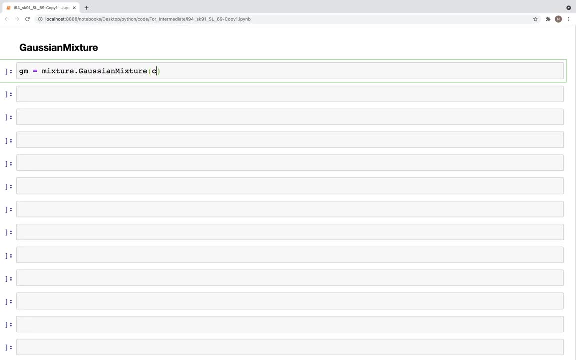 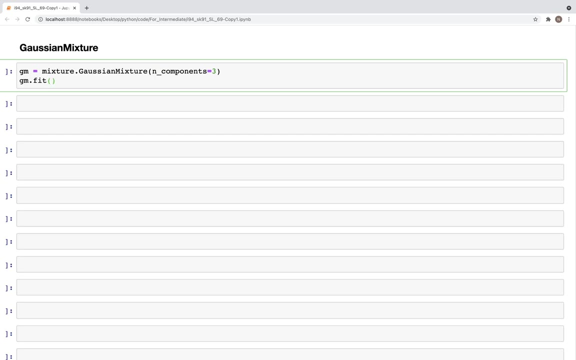 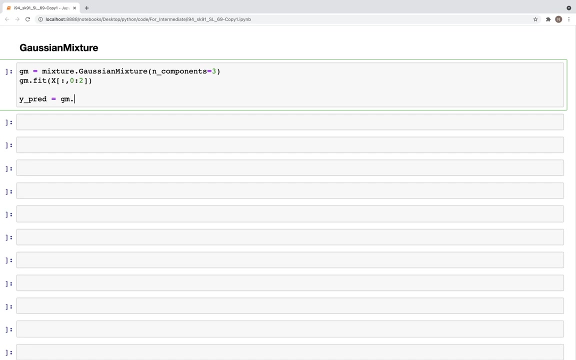 Gaussian mixture and- and we'll specify the end components- is equal to three gm dot fit, and this would be on just the all the records, but then just the first two columns and we can put the predicted values in here in the y pred gm dot predict, and these would now have cluster labels attached after the prediction is done. so 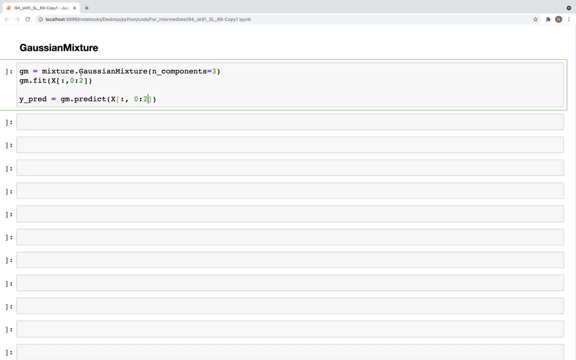 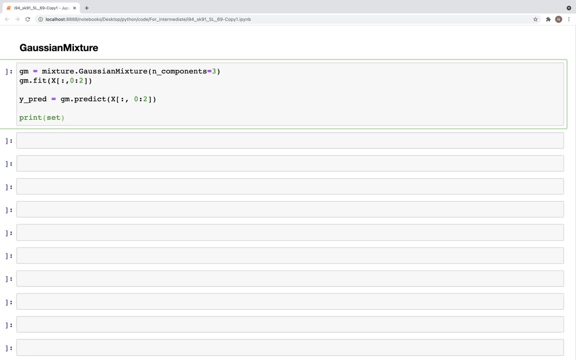 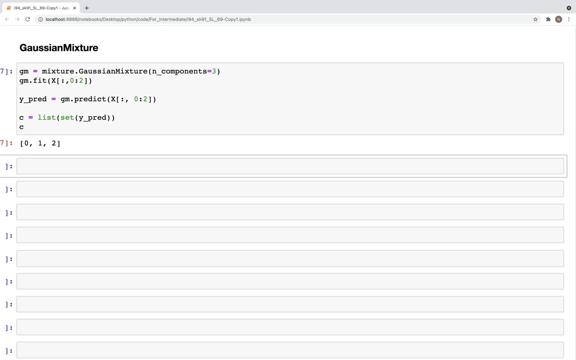 we can use them for plotting 0 to 2 and we can print the set for. so let's call this: c is equal to list, set of y, underscore pred, and then we can look at c. so we have three classes: 0, 1 and 2, after the fit was done on x. so here point to note is we do not have 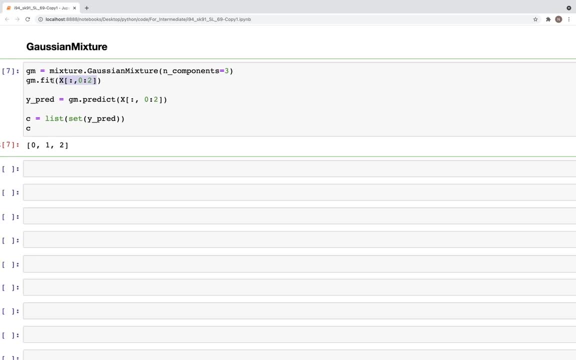 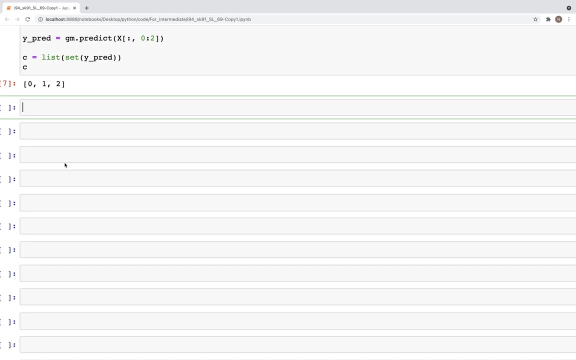 the y target in here in the fit method that we usually have for supervised case. now let's perform, let's plot this so: c 0- i'm going to separate them out into different, uh, uh, different arrays: c 0, c 1, c 2. this would have label 0 and we go from 0 to 2 and i'm going 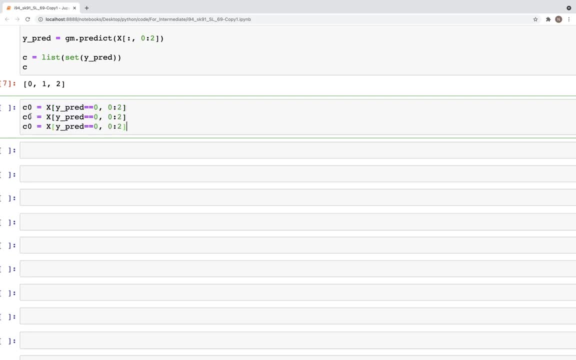 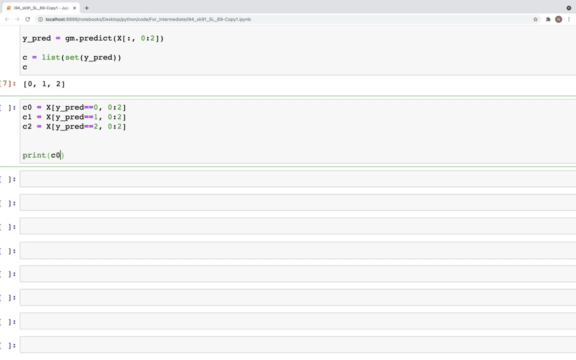 to copy this. paste it two times, because this would be the class one, this would be correct, and the class 2 would be: uh, class 1.. class two and then this would be one, this would be two. so those are the classes. you can print these zero dot shape. see one dot shape and see two dot. 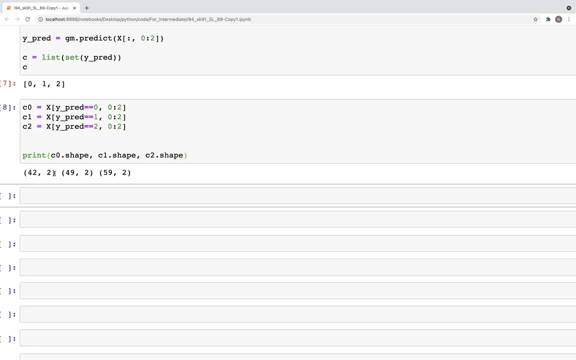 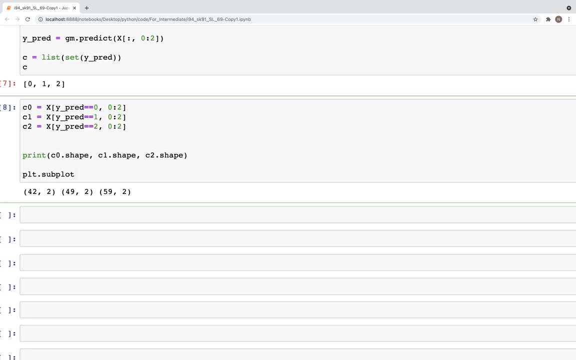 shape and we have about unequal, about still 42, 49 and 59 data points in each of those clusters. you can now plot all of this, so PLT dot subplot and I'm going to create subplot so we can easily compare the original and the predicted. 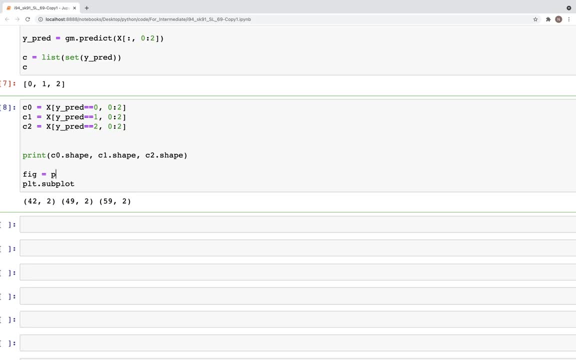 side-by-side. so figure is equal to PLT dot figure. big size is equal to, let's say, 15 by 5 and we have top plot. we just need one row, two columns and three columns next to the third column. these are little squares and we have 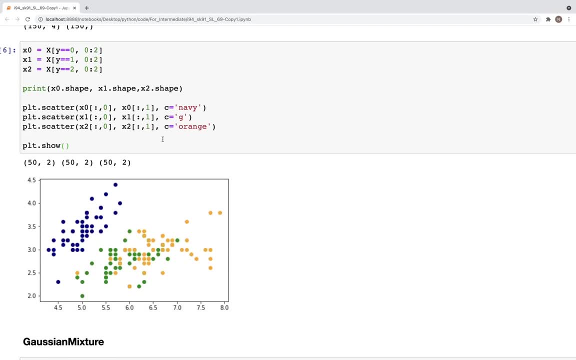 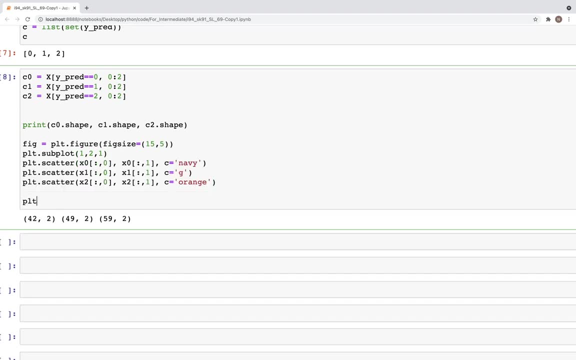 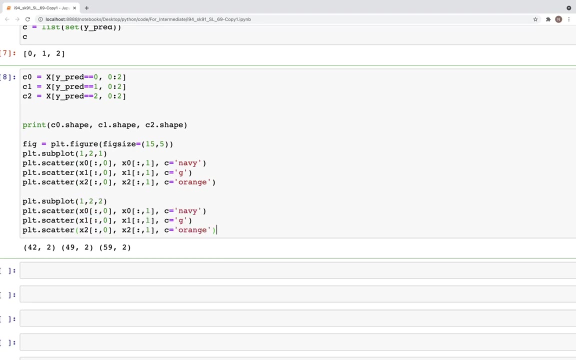 plot number one: on the left hand side we'll put this original plot that we have above and then down below. uh sorry, on the right hand side we can put the second plot one, two comma two, and there instead of c x we have c. oh, let's change that small c and change this here. 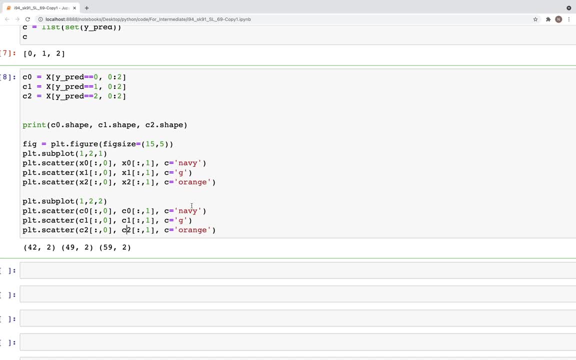 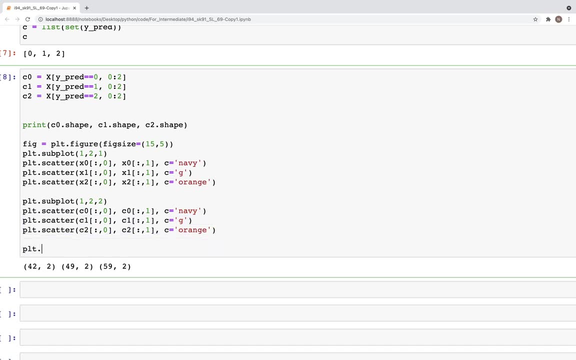 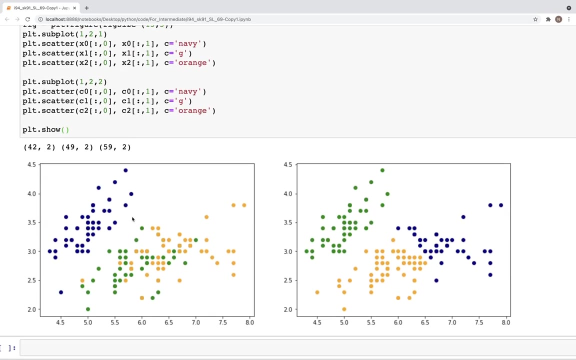 and this and this now point to remember is that these colors here may not exactly match what we have above, so we can change that later. plt dot show and here we have. these colors are. so the blue should be green, the green should be orange. uh, the green should be orange now. 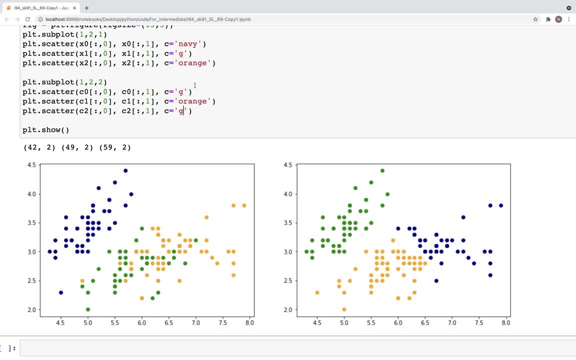 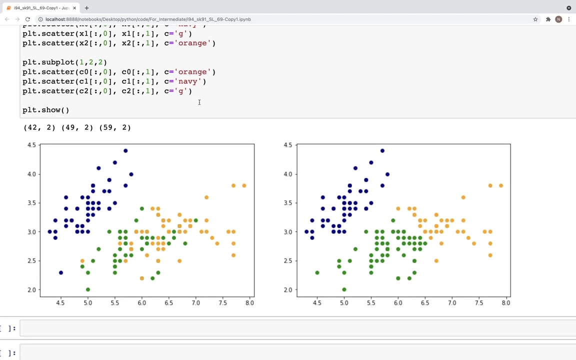 the orange should be orange, now should be green, the green should be blue and the blue should be orange. okay, uh, this should be orange, the green is good and this should be blue now we should. okay, so, as we can see, it was able to identify this blue cluster, uh. 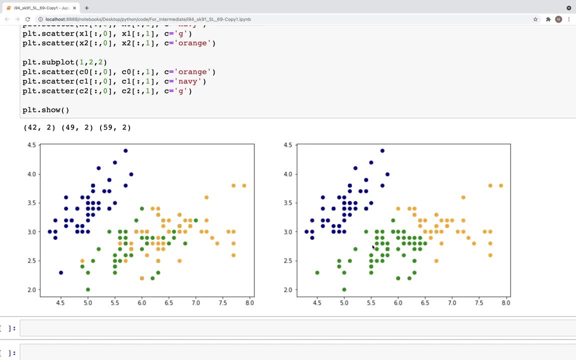 so, as we can see, it was able to identify this blue cluster, uh, accurately, but there is overlap in this particular accurately, but there is overlap in this particular accurately, but there is overlap in this particular green and yellow cluster. so it was able to green and yellow cluster. so it was able to. 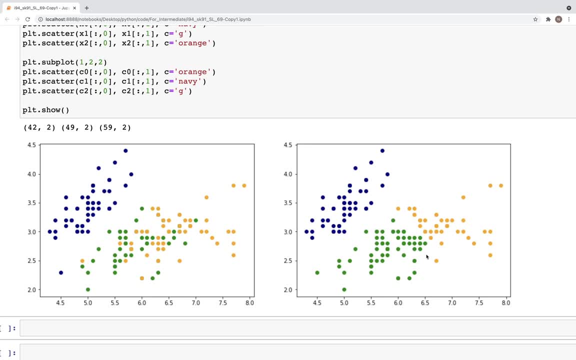 green and yellow cluster, so it was able to identify these, identify these, identify these. now, here we are. uh, the way we are plotting. now here we are. uh, the way we are plotting. now here we are. uh, the way we are plotting. we are not plotting or coloring these based. 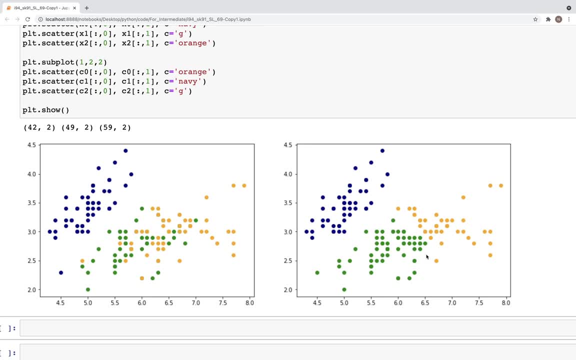 we are not plotting or coloring these based we are not plotting or coloring these based on the priorities. if we had we colored on the priorities, if we had we colored on the priorities, if we had we colored based on priorities, we would see. based on priorities, we would see. 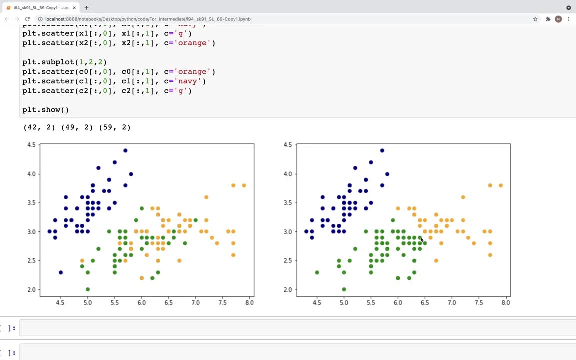 based on priorities, we would see. part of these could be yellow and part part of these could be yellow and part part of these could be yellow and part of these could be green. of these could be green. of these could be green, especially in the area where there is. 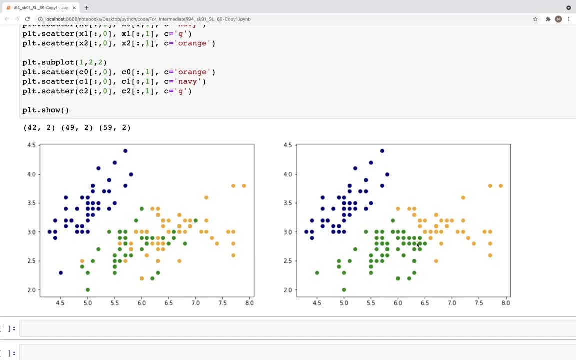 especially in the area where there is, especially in the area where there is overlap, but here this looks like a overlap, but here this looks like a overlap, but here this looks like a um, a hard, um, a hard, um, a hard margin. uh, instead of a soft margin. 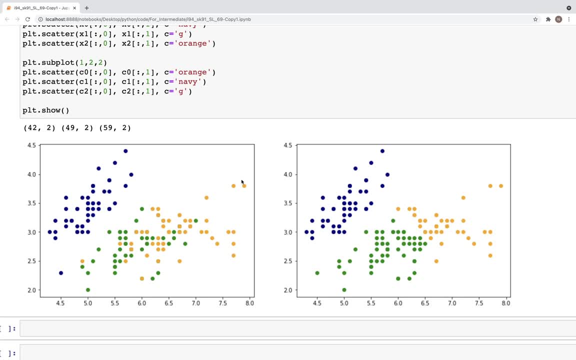 margin: uh instead of a soft margin. margin- uh instead of a soft margin. but we can get uh predicted, but we can get uh predicted, but we can get uh predicted. priorities as well, and to the plot priorities as well, and to the plot priorities as well, and to the plot uh. next, let's look at the bayesian. 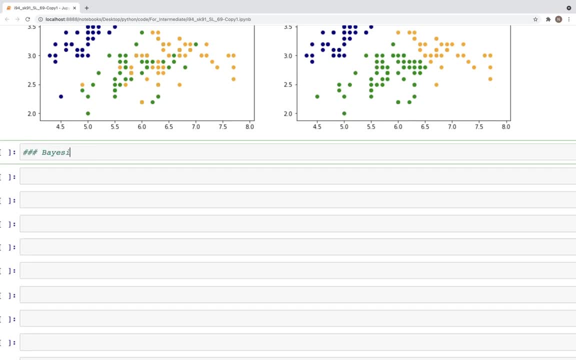 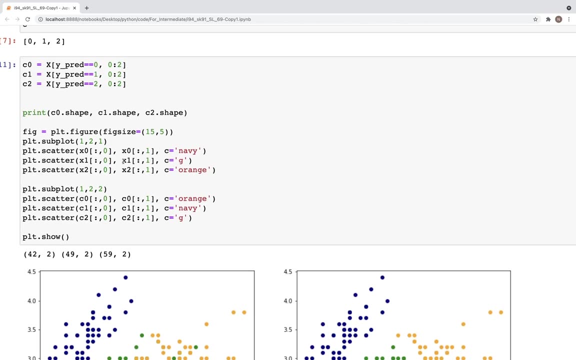 uh. next, let's look at the bayesian? uh. next let's look at the bayesian approach of this. so, approach of this, so approach of this. so bayesian, bayesian, bayesian, gaussian mixture, gaussian mixture, gaussian mixture, and and and. for this i'm going to copy. 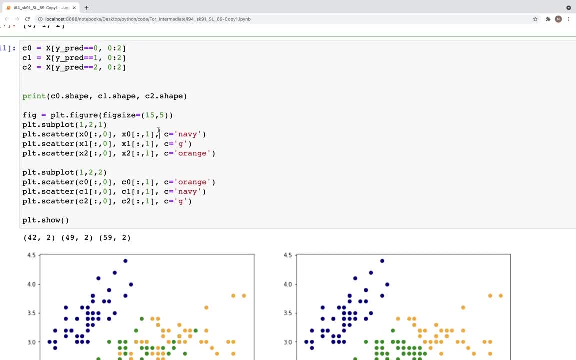 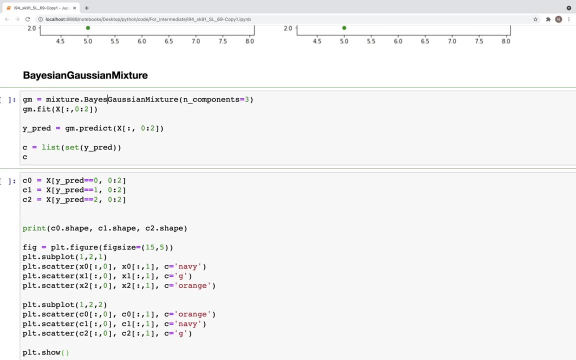 for this. i'm going to copy, for this. i'm going to copy on the same code, on the same code, on the same code, down here, for down here, for down here, for uh model and for the plots. uh model and for the plots. uh model and for the plots. so here, all we need to do is add bayesian. 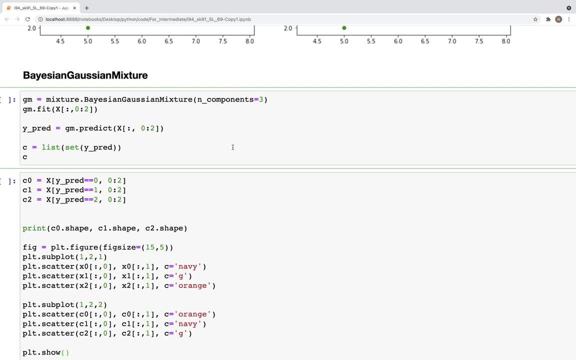 so here all we need to do is add bayesian. so here all we need to do is add bayesian. and for the number of components, and for the number of components, and for the number of components: uh, i tried, uh, i tried, uh, i tried plotting without. 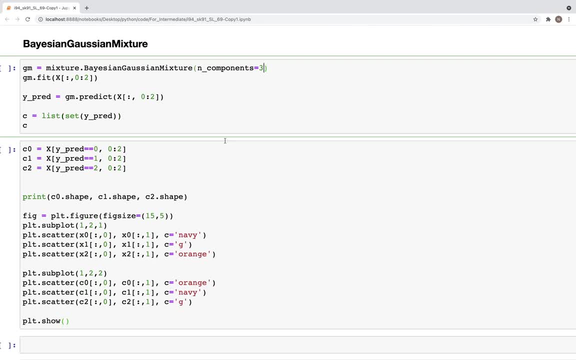 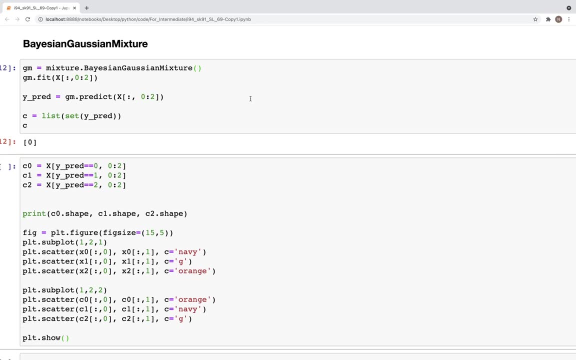 plotting without plotting without uh this, but that, uh this, but that, uh this, but that gives a, gives a, gives a, gave a wrong results, gave a wrong results, gave a wrong results. so let's say, if we remove this, so let's say, if we remove this, so let's say, if we remove this, we just get one component, as you can. 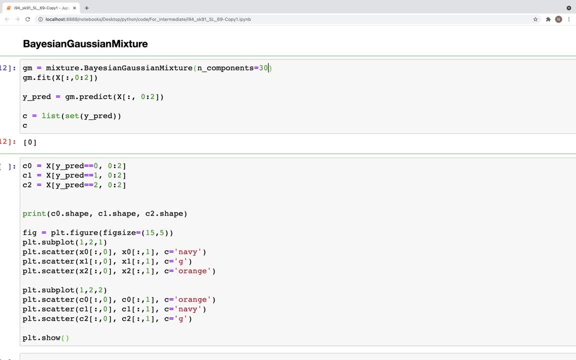 we just get one component, as you can. we just get one component, as you can see, that's the zero, see, that's the zero, see, that's the zero. so if we put 30 in there and now we get, so if we put 30 in there and now we get, 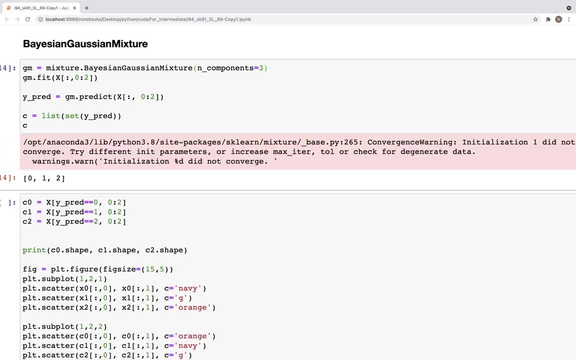 so if we put 30 in there and now we get three components, i've uh continued with just uh three. i've uh continued with just uh three. i've uh continued with just uh three: components, components, components, and that that works just fine, and that that works just fine. 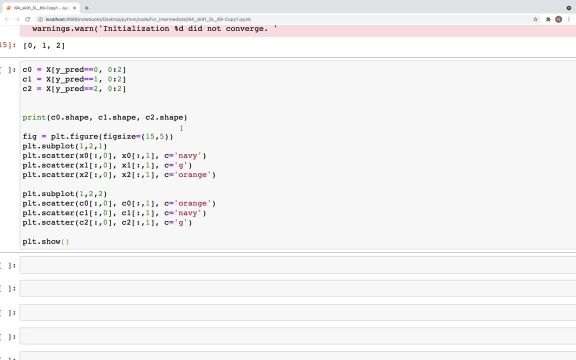 and that that works just fine for this case. so with those three for this case, so with those three for this case. so with those three components, we can again go down here. components, we can again go down here. components, we can again go down here and perform the fit. 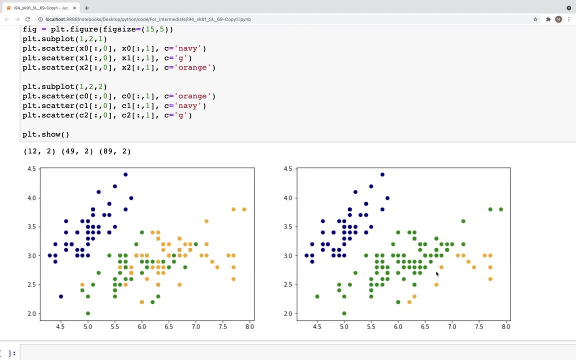 and perform the fit, and perform the fit, and, as we can see, and as we can see, and as we can see, the fit is not as good, so the the fit is not as good, so the the fit is not as good, so the overlap, overlap, overlap area is not. 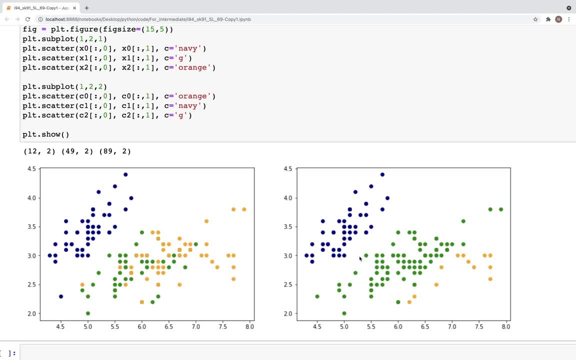 area is not, area is not found correctly, found correctly, found correctly, and and and that's that's. that's one of the reasons could be that these, one of the reasons could be that these, one of the reasons could be that these points are so close, that points are so close that 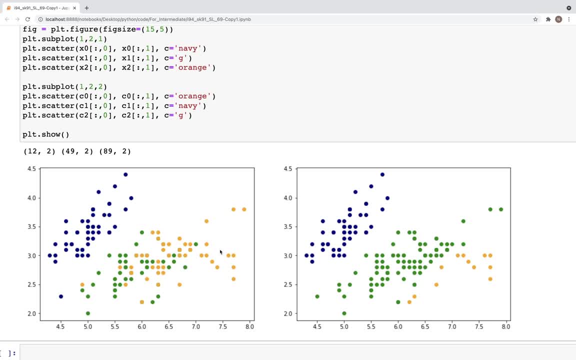 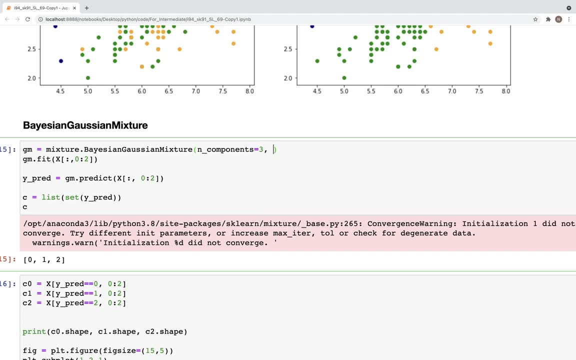 points are so close that, uh, uh, uh, it could just be one cluster there, it could just be one cluster there, it could just be one cluster there, now, now, now, this could be optimized, this could be optimized. this could be optimized. um, um, um, one, um, one, um, one, uh. item that we can change here is the: 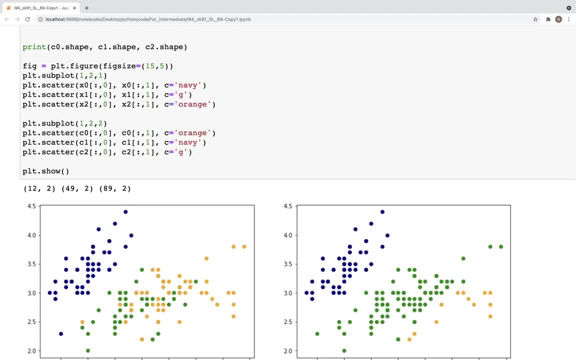 uh item that we can change. here is the uh item that we can change. here is the tolerance. so if we set the tolerance to tolerance, so if we set the tolerance to tolerance, so if we set the tolerance to 0.1, 0.1, 0.1 and run this again, we see that we now 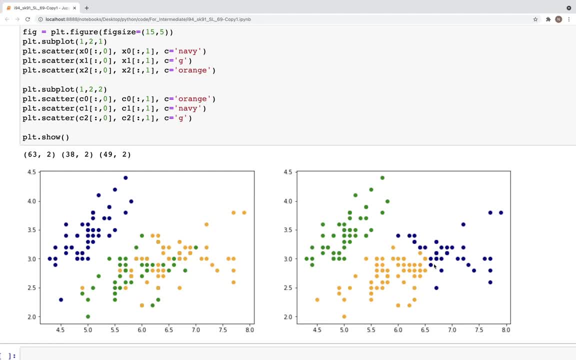 and run this again. we see that we now, and run this again, we see that we now can, can, can this, this, this: find those clusters that are overlapping, find those clusters that are overlapping, find those clusters that are overlapping, if you go, if you go, if you go further, more maybe 0.2. 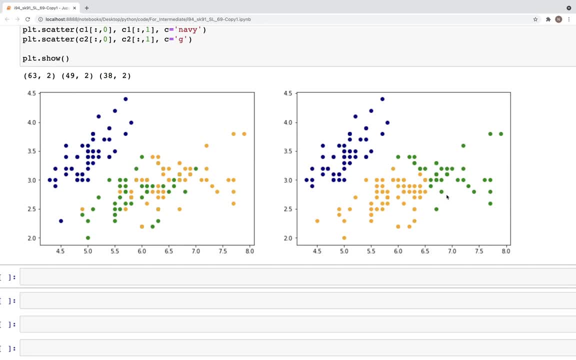 further more, maybe 0.2, further more, maybe 0.2, and run this again. so now we have most and run this again. so now we have most and run this again. so now we have most of these, of these, of these, and that's similar to what we had. 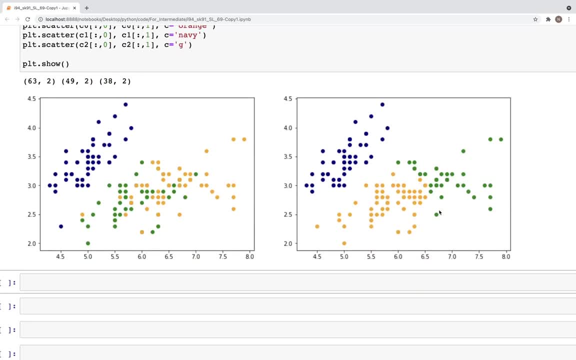 and that's similar to what we had, and that's similar to what we had earlier. so these plots earlier, so these plots earlier. so these plots, these data points, these data points, these data points, uh uh, uh. that was it then for this video. i hope in. that was it then for this video. i hope in. 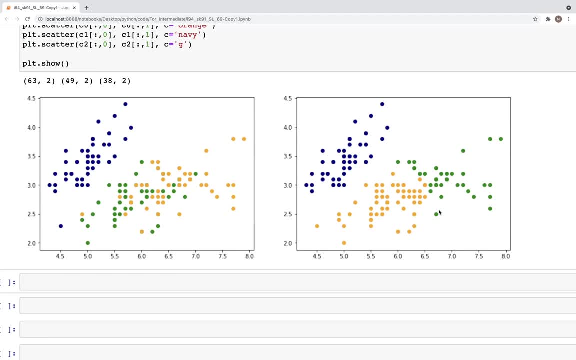 that was it then for this video. i hope in this video and previous series of videos, this video and previous series of videos, this video and previous series of videos on intuition, you now have on intuition. you now have on intuition. you now have, uh, some experience, hands-on experience. 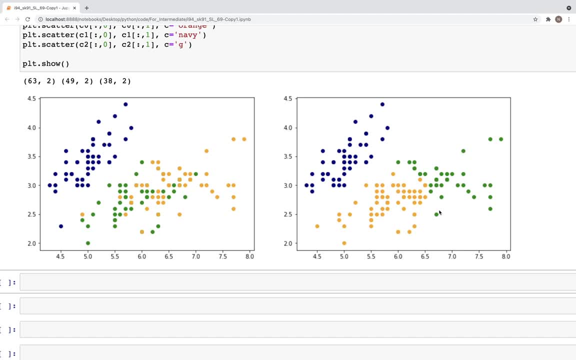 uh some experience, hands-on experience. uh, some experience, hands-on experience on how to implement gaussian mixture. on how to implement gaussian mixture. on how to implement gaussian mixture models, models, models. uh. bayesian gaussian mixture models. uh. bayesian gaussian mixture models. uh. bayesian gaussian mixture models. uh. on artist: tired toy data sets.